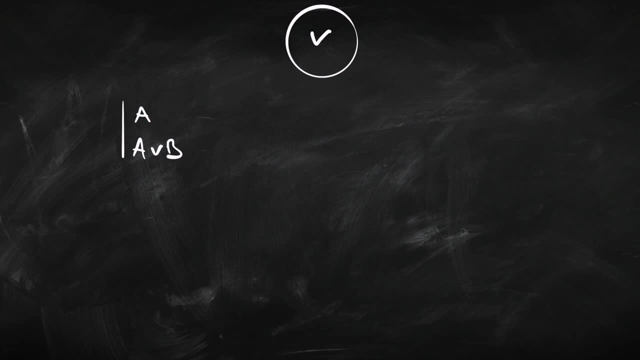 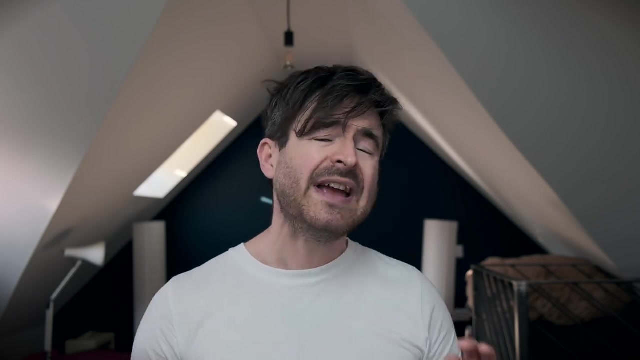 have A in a proof, we can introduce disjunction, So A or B, And we can also do it the other way round. So if we have A, we can introduce B or A. These are the or introduction rules. The elimination rule for or is a little bit more complicated, So let's go through this one slowly. 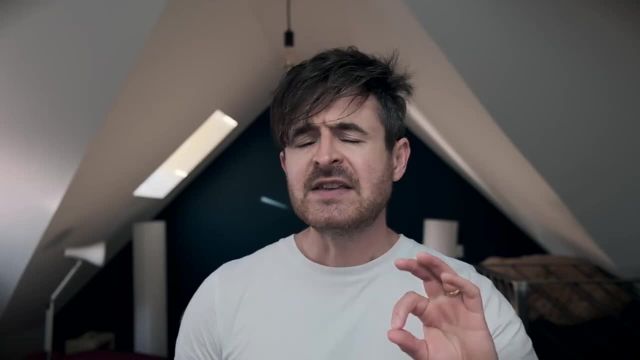 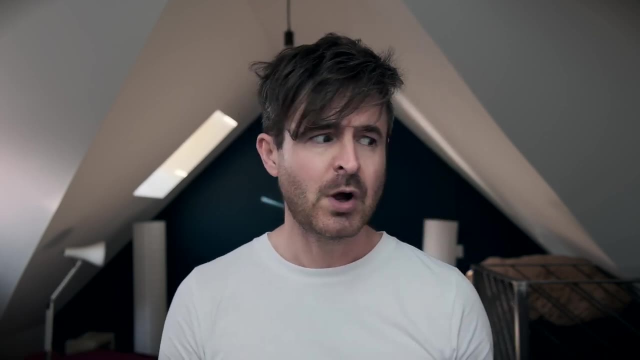 Suppose we've got A or B in a proof. Okay, there's no obvious way that we can swiftly eliminate that, because if A or B is true, we don't know which one. it is. Okay, we don't know that A is true, we don't know that B is true, So we can't go directly to A. 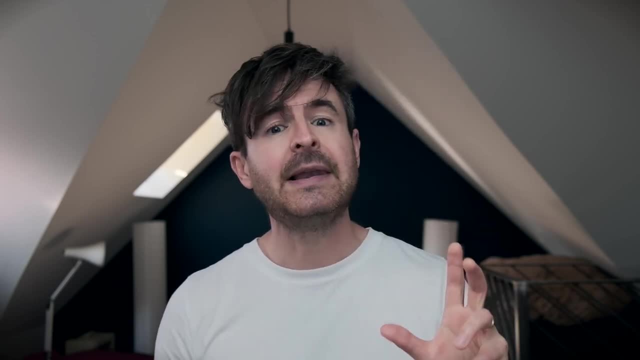 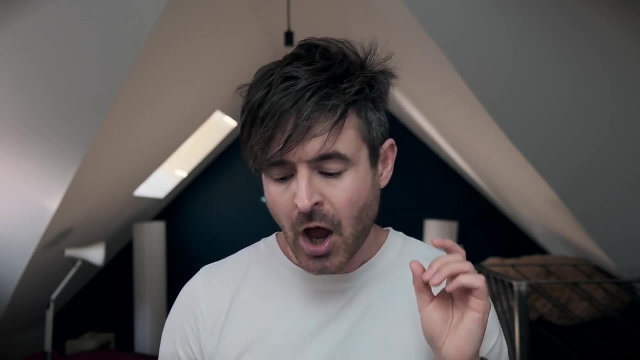 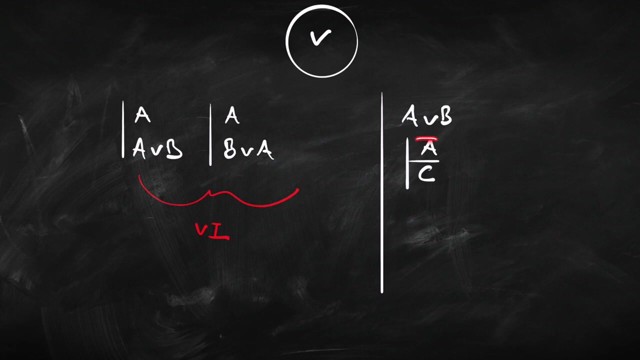 we can't go directly to B. We have to do something a little bit trickier. So what we can do is, in effect, a bit of side working with some embedded sub proofs. Okay, so we know that either of A or B is going to be true, So suppose we assume A and conclude some third thing, C, And then also. 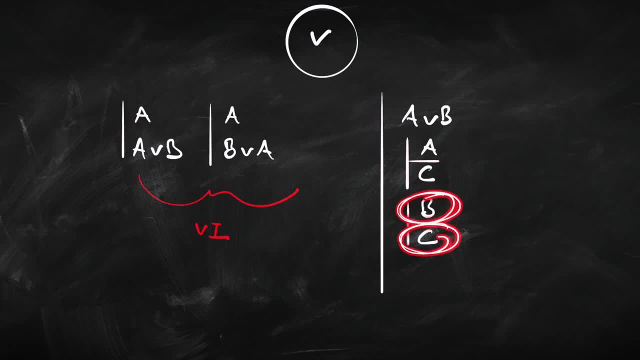 we assume that B, and we conclude the same third thing, C. So what we've done there is we have said: well, if A is the case, then so is C, And also, if B is the case, then so is C. Okay, so C follows from. 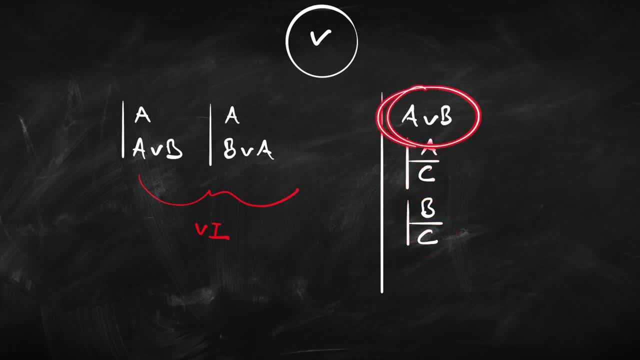 A, C follows from B, and we know that either A or B is the case, So either way, C is going to follow. This is the elimination rule for disjunction. Okay, so let's go through it again, because it's a bit more complicated. If we start off with A or B, what we do is assume A. 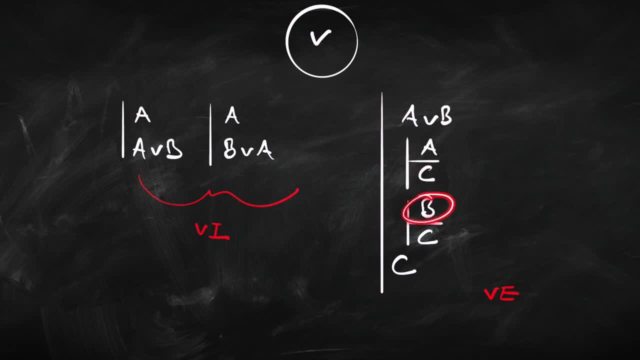 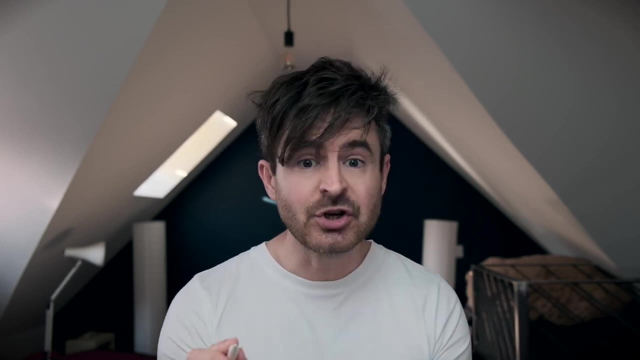 derive C and then independently assume B and derive that same thing, C. The C here and C here have to be the same. If we can do that, then we can say that C on its own follows from A or B. Let's have a look at the arrow, the conditional for if, then It's introduction rule. we've already. 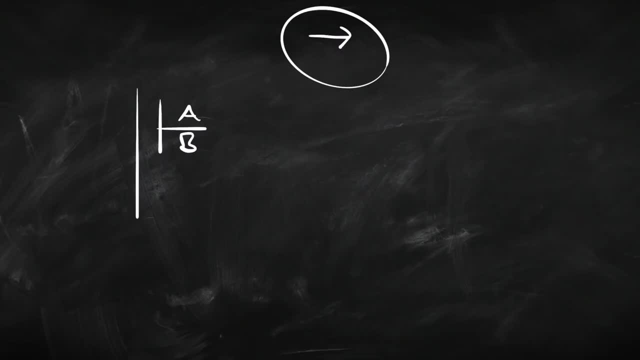 met in the previous video via conditional proof. If we assume A and can derive B from that, then we can introduce: if A, then B, outside the scope of that assumption. Okay, so to reiterate that we assume A, derive B and then cancel that assumption and infer if A then B. That is the. 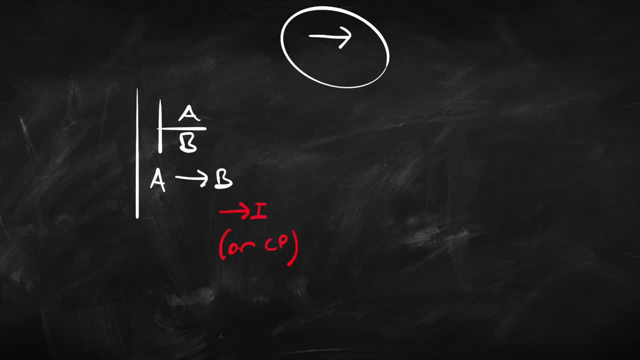 introduction rule for the arrow, or it's also known as conditional proof, The elimination rule for the arrow. we've already met that too. If we have premises, if A, then B and also A, we can infer B, That one's modus ponens. Okay. so we can either call it the arrow elimination rule, or we can call 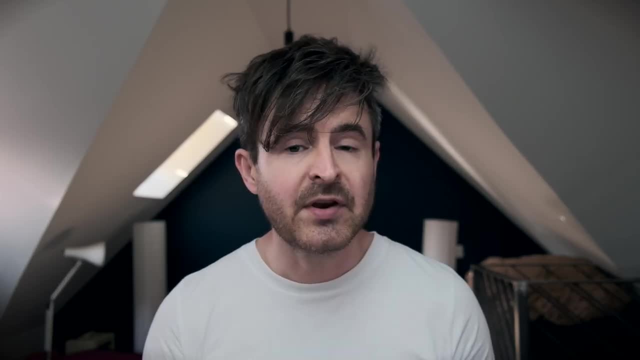 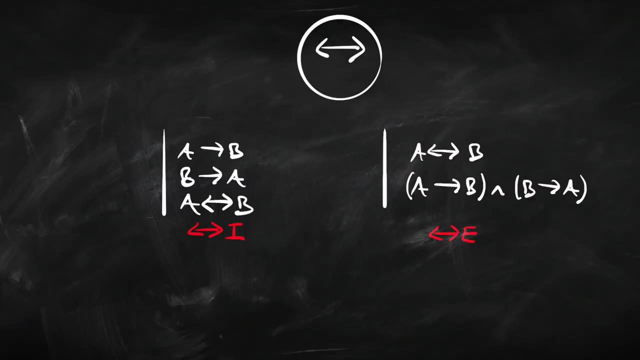 it modus ponens In the case of the biconditional if, and only if. well, we don't have any special rules here, We kind of just treat it via its definition, with the arrow. So to introduce it into a proof, if we have an arrow going one way and an arrow going the other way, then we can. 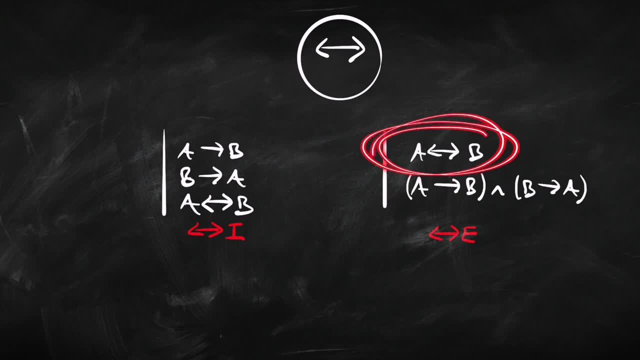 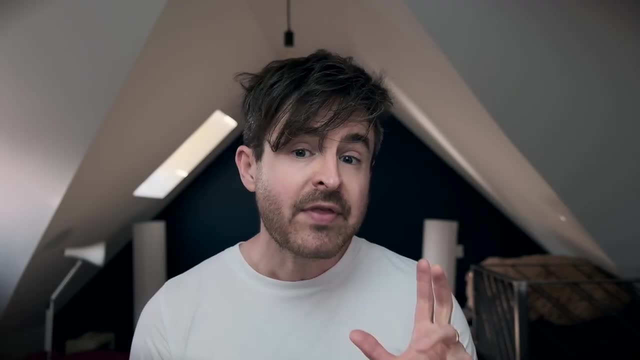 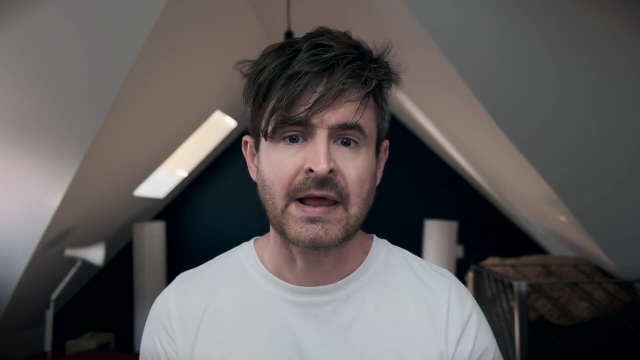 introduce the two-way arrow, And if we have the two-way arrow in a proof, then we can infer via its definition, to A An arrow going one way and the arrow going the other. So there, we've looked at all of the connectives apart from negation, And negation is going to be a little bit more complicated. 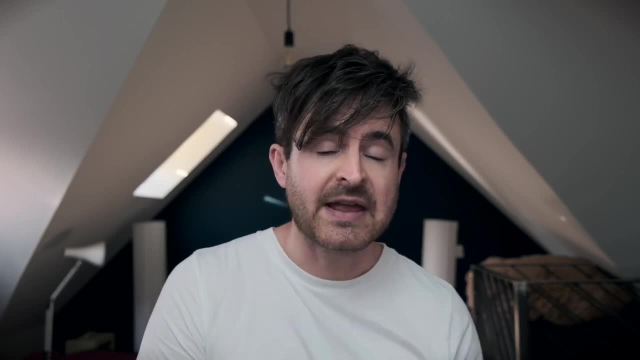 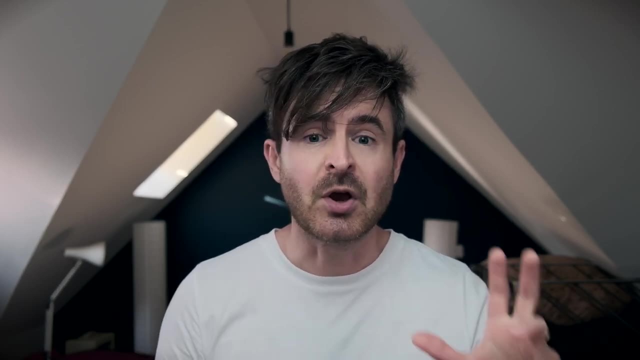 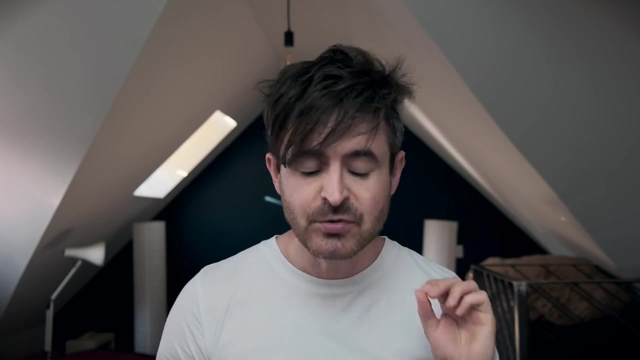 And, in fact, there are different ways of reasoning about negation in natural deduction. There are different options for us in selecting which rules we're going to use, So I'll explain the rules that we're going to use In order to reason about negation. we're going to introduce a new device. 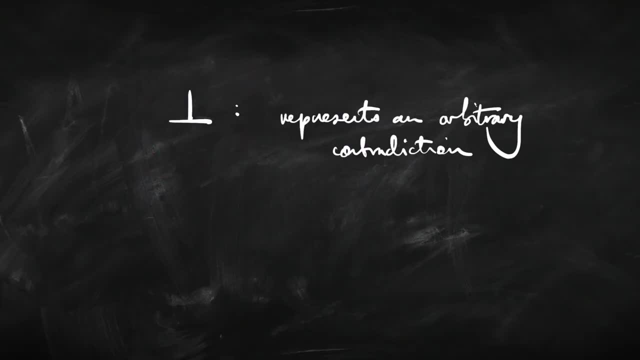 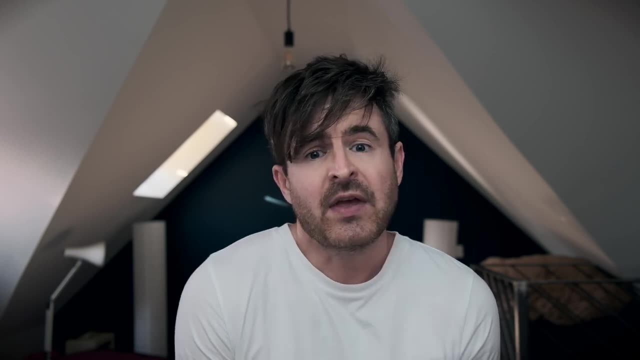 This gun, This guy here sometimes called fulsome, It's like an upside down T And it's going to represent for us an arbitrary contradiction. So you could think of this as P and not P or whatever, But we're going to use 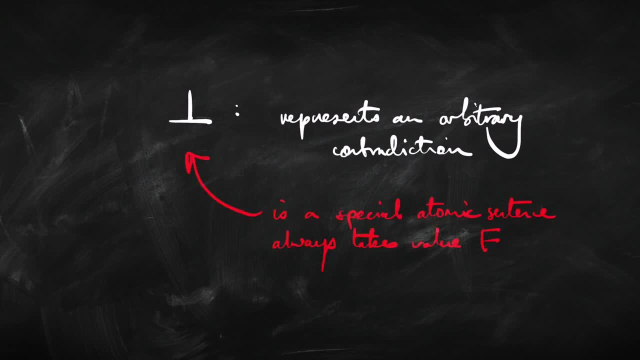 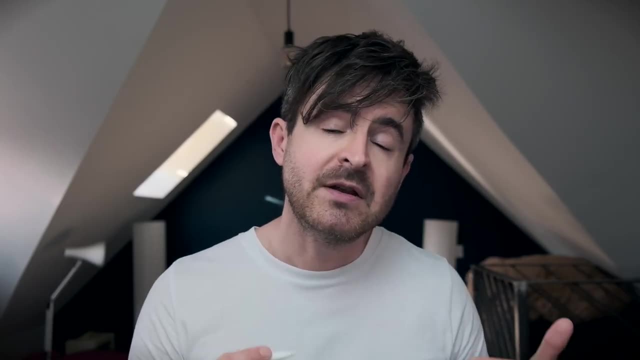 this symbol. It's a special kind of atomic sentence And it always takes the true value false. How does it help? Well, it helps us formulate nice rules for negation. Let's have a look, Okay. so our first rule allowing us to: 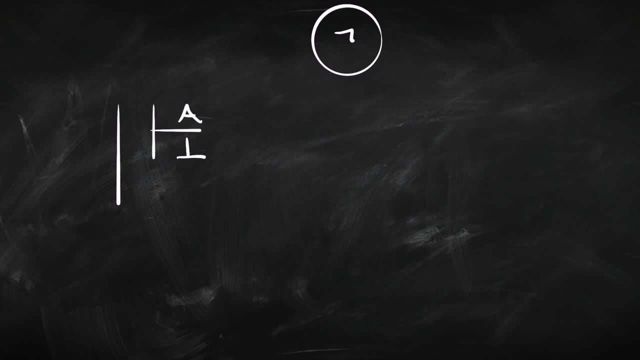 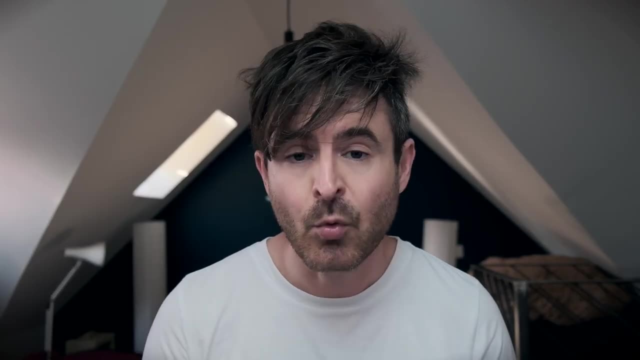 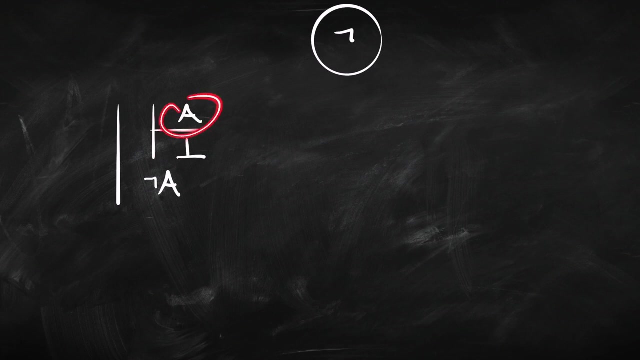 introduce negation goes like this: Suppose you assume something, A, and you can derive a contradiction from it That indicates that something went wrong with that assumption. The assumption must have been wrong. So what you can infer is not A You assumed A, You showed that. 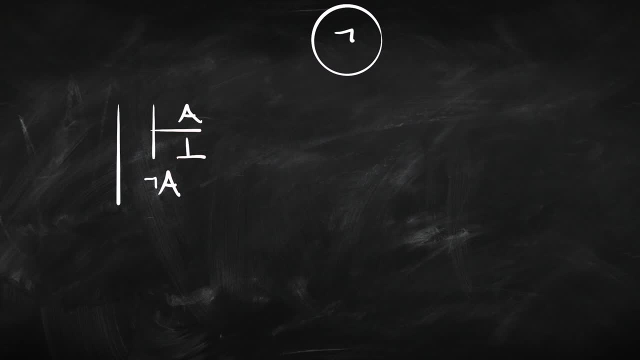 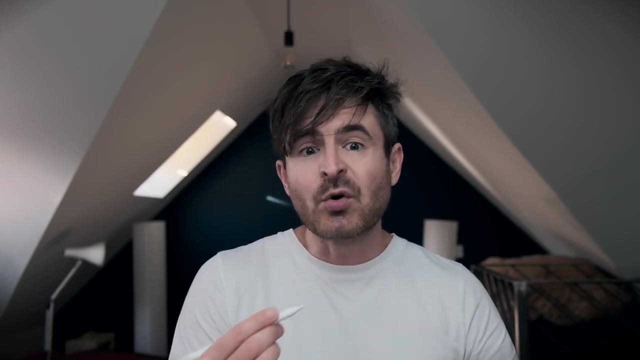 that can't be right. So you can infer: not A. So this is our way of introducing negation. It's our negation introduction rule, But we can also call it by its name: Reductio ad absurdum. Okay, now we're going to hear that term quite a bit. It's a way of inferring. 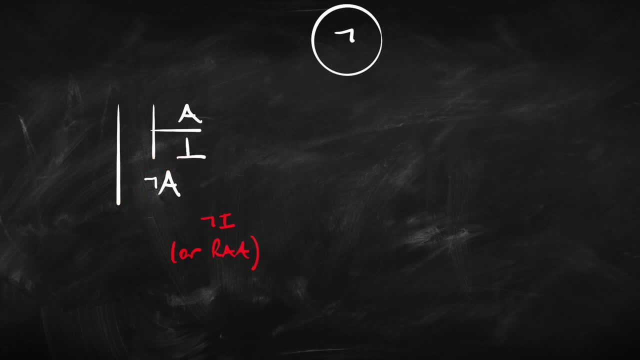 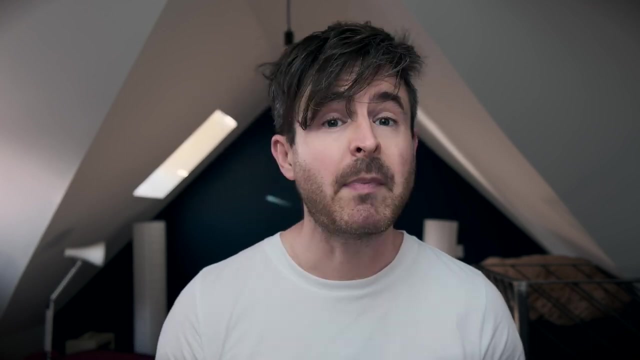 that something isn't the case. What you do is you first of all assume that it is the case And then you show that that can't possibly be right by deriving a contradiction, And then you infer the negation of that thing. Okay, reductio ad absurdum, So that's our introduction rule for negation. What about the? 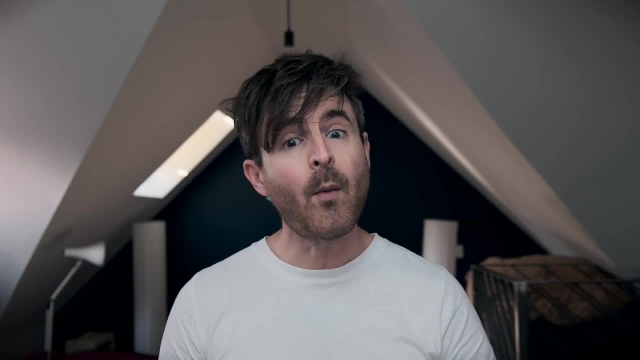 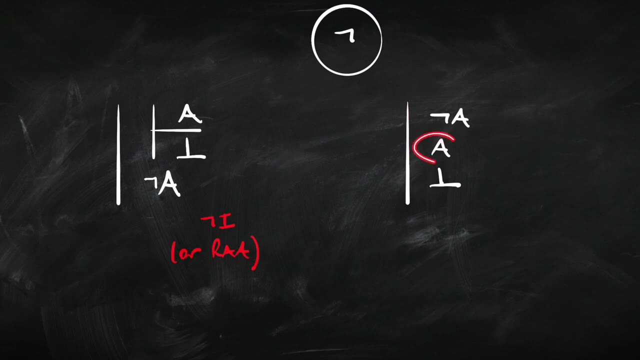 elimination rule. Well, here we have some options, But the one we're going to use is the elimination rule. So what we can do is this: Suppose we have not A in a proof And suppose we can also demonstrate A, In other words, we can get a contradiction going there. Well, in that case we can introduce: 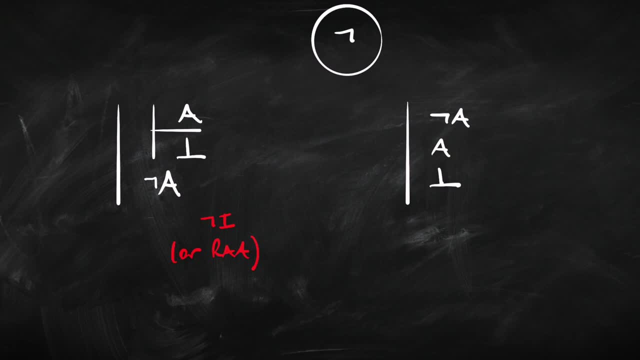 our Folsom constant. Okay, because this is our, it's like our marker for a contradiction. So if we start off with not A and we turn it into a contradiction, we can introduce the Folsom constant. So this is our elimination rule for not, But we could also call it the introduction rule. 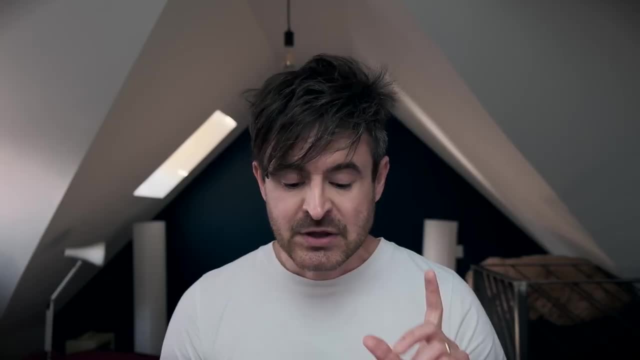 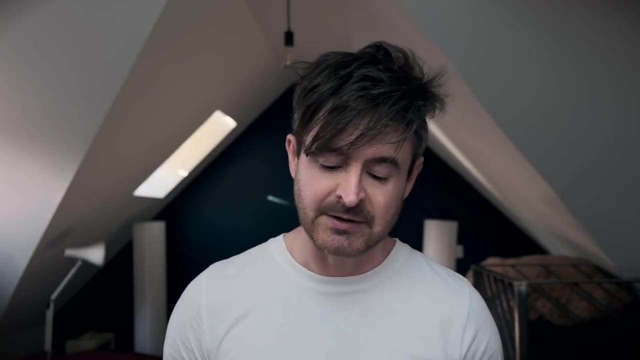 for the Folsom constant. So this is our elimination rule for not, But we could also call it the. either way. really, Now, because we've introduced this new primitive sentence, the Folsom, into our language, we're going to need some rules for it. These ones don't quite. 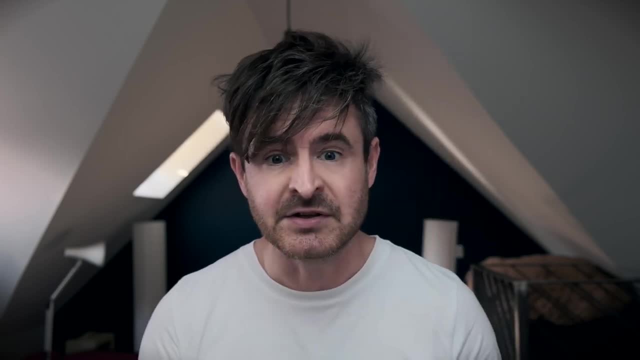 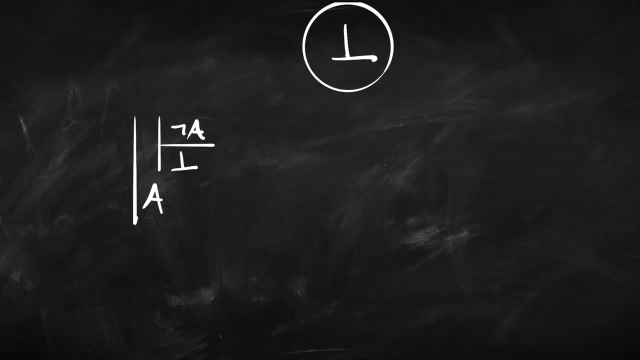 correspond to the introduction elimination rule paradigm. Let's have a look at the two rules for the Folsom constant. The first one looks a little bit like our reductio ad absurdum rule, but it's different. It says: if we start off assuming that A is false, not A, and we get a contradiction. 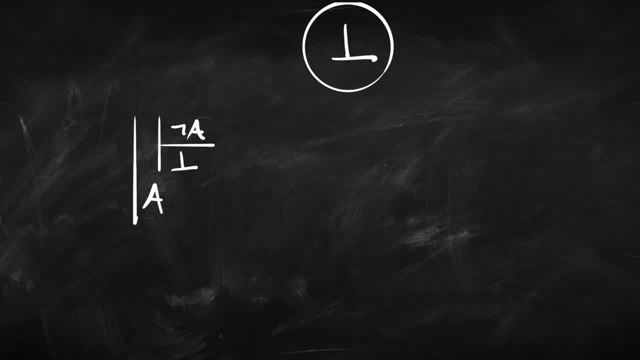 from that our Folsom constant. well then we can infer A. Okay, so if we assume that something isn't the case and we're proved wrong, it must be the case- We infer A. That's known as indirect. 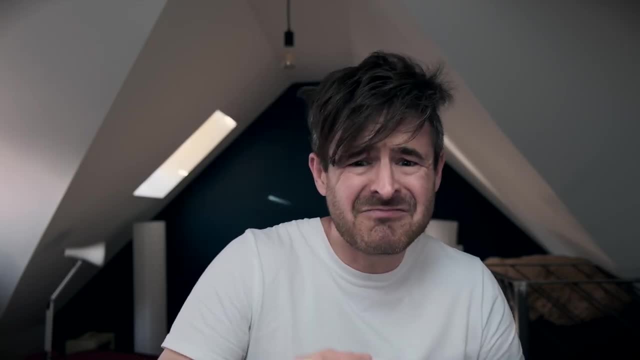 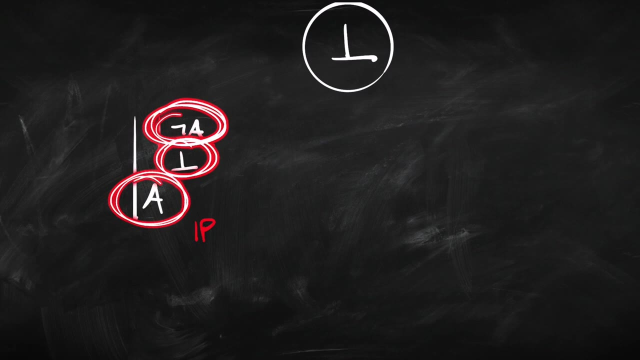 proof. It's called indirect proof because you kind of go around the houses a little bit, You're assuming that something is false, getting a contradiction and inferring that is in fact true. So that's one rule for Folsom. Here's the other one, Really simple. 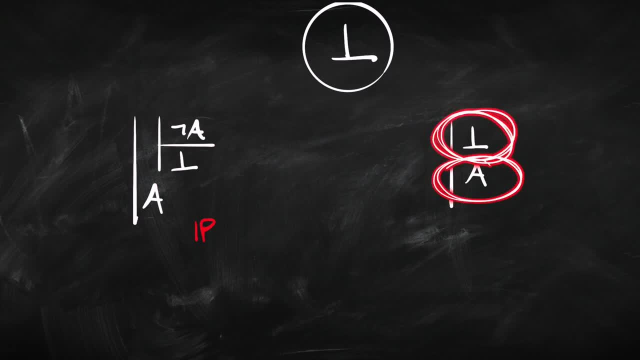 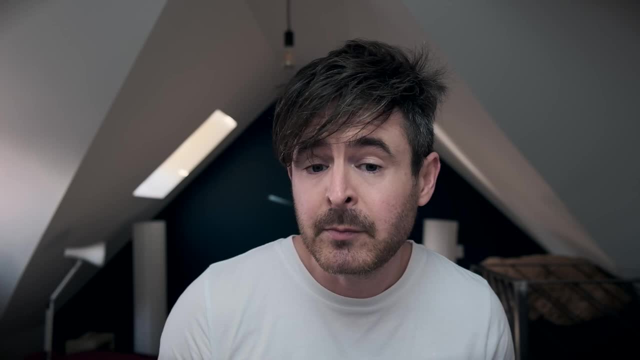 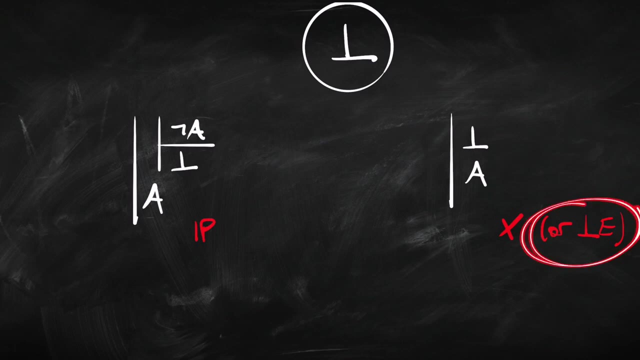 From the Folsom constant you can infer any old sentence you like. There are lots of different names for this rule. Some people call it X-Falso-Quadlibet. From a contradiction or from a falsehood, anything follows. We're just going to call it X, Or you could call it Folsom. 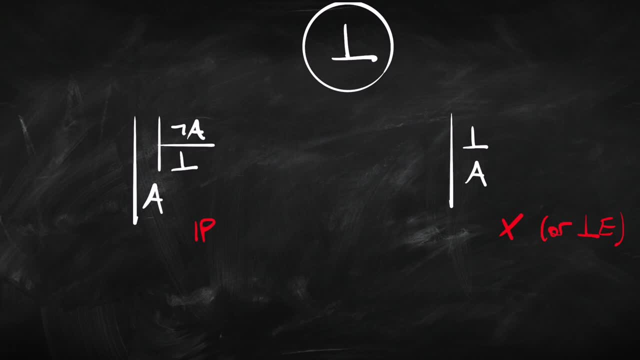 elimination. Okay, now that rule might be a bit confusing. Okay, why should it be that A, any old sentence A can be concluded from a contradiction? Well, think about our definition of entailment. using truth tables, Entailment says it can't be that. the premise is: 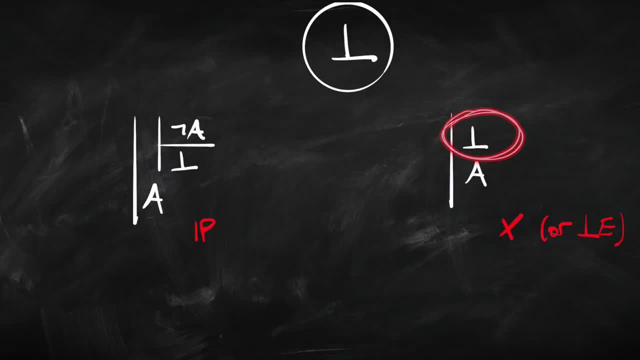 true and the conclusion is false. But this chap can never be true. So it can never be the case that this is true and this is false. So this inference is always going to be a good one. whatever A is, A could be as absurd as you like, It's always going to follow from this. 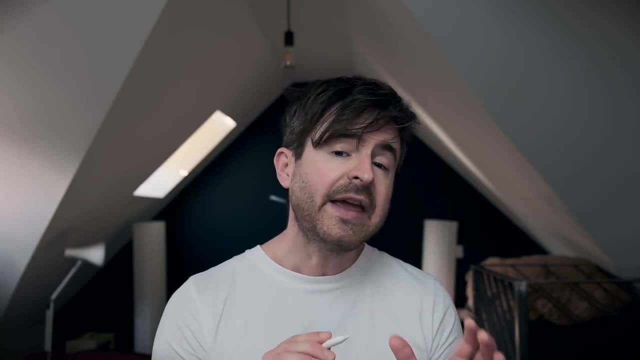 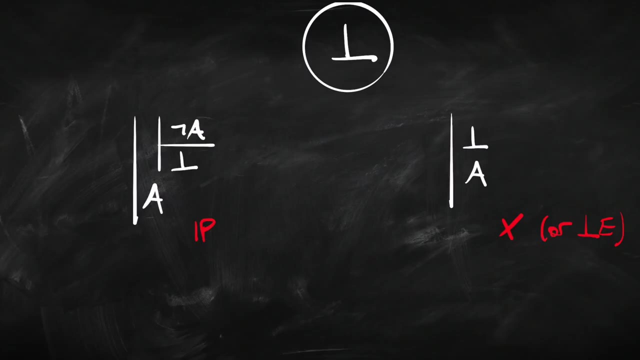 because this can never be true. Okay, like I said, there are different ways of formulating these rules for negation. There are different ways of formulating these rules for negation. We have picked two rules for negation plus two rules for Folsom. We could have picked a different. 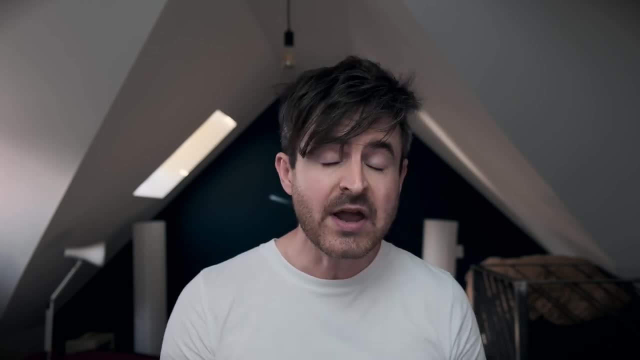 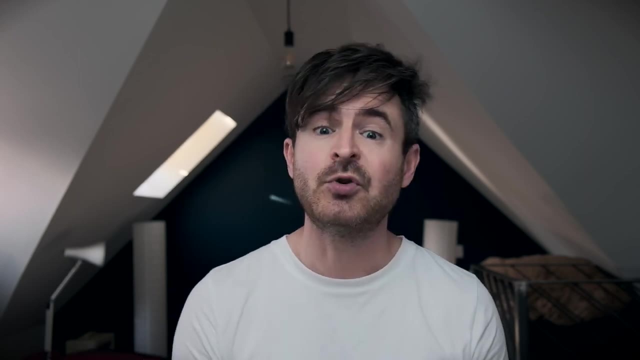 set, And later on in the next video we're going to look at some different rules for negation and we're going to show how they're interchangeable. In fact, using the rules that we've got here, we can derive those other rules. That's the sense in which it doesn't really matter which ones we 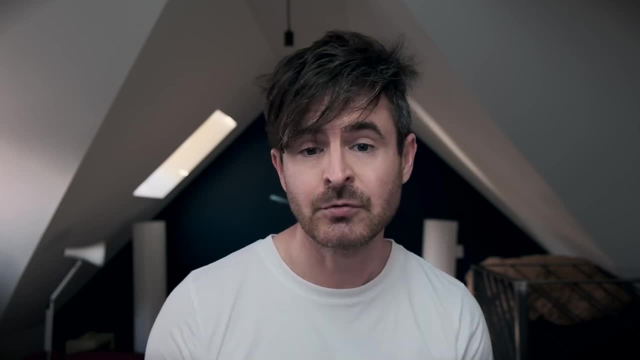 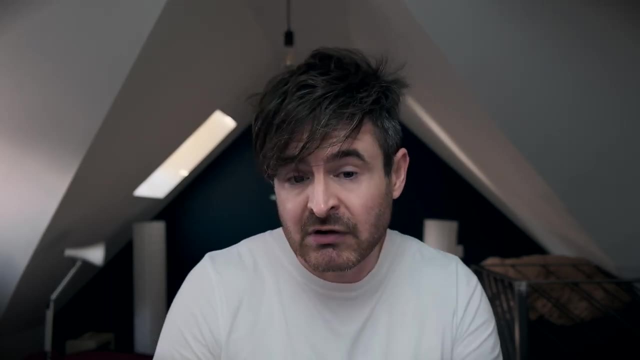 pick. But what does matter is that we pick a fixed set of rules and we say: we're going to learn these, we're going to get comfortable with them. So there are the rules for Fitch-style natural deduction, or at least the rules that we are. 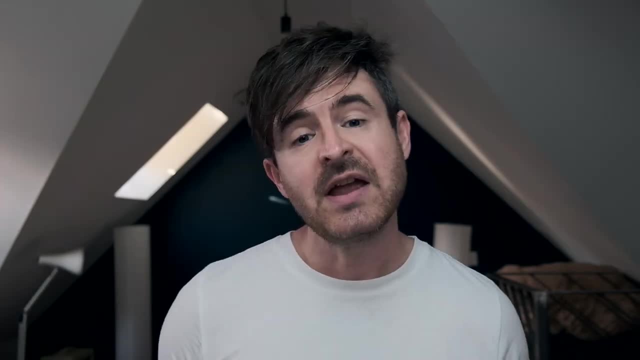 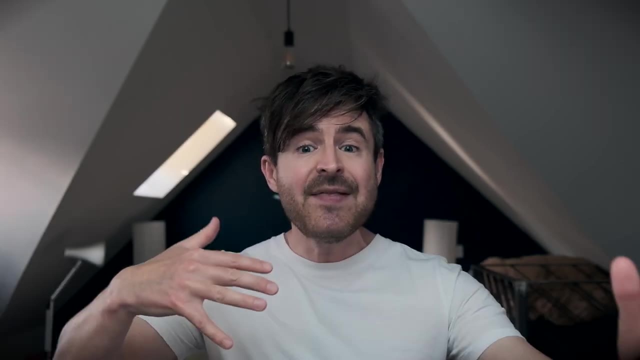 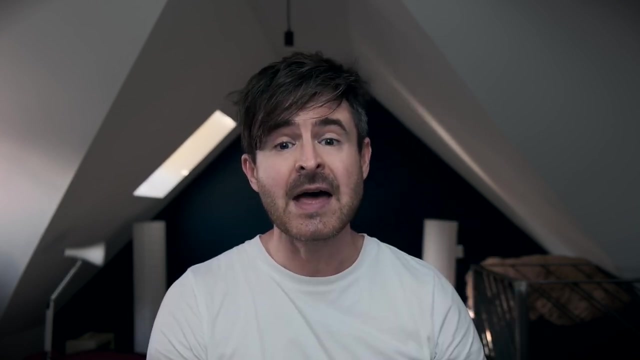 going to work with for propositional logic. Okay, guys, that is all for this brief introduction to the rules that we need for Fitch-style natural deduction. In the next video we are going to look at how we use those rules to construct Fitch-style proofs. Stick around for that.